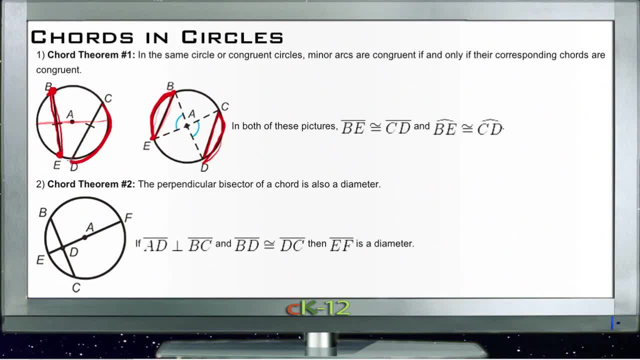 that, say, CD over here, the arc was congruent to BE this arc over here, then we would also know that those corresponding chords were then congruent as well. So across two different circles or within the same circle. Our second theorem is that the perpendicular bisectors 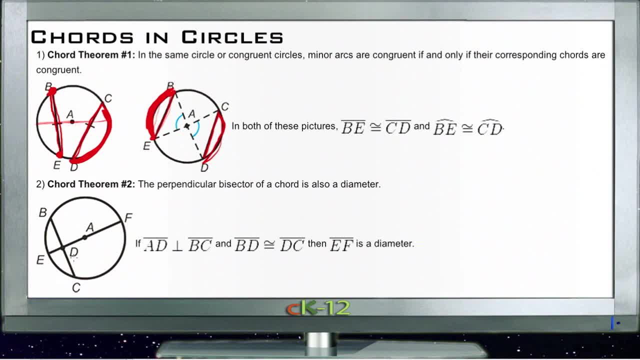 the bisector of a chord is also a diameter. Now this makes sense if you think it through. No matter how long a chord is, if we take any two points on a circle and we connect them with a line, no matter how long that line is or how far apart they are on the circle. 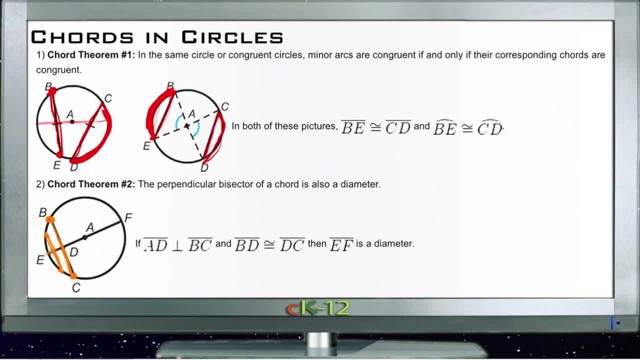 if we draw a line that's perpendicular to them, then that line is going to have to be going through the center of that chord. If it goes through the center of that chord, making it a bisector, and if it's perpendicular to that chord, then it's going to go right through the center. 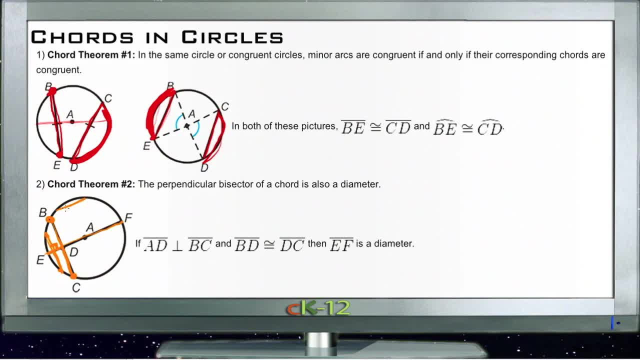 of the circle every time. If we do a shorter one over here, if we bisect it at the center- and this is 90 degrees right here- then this line that we're making will go right through the center of the circle. So the perpendicular bisector of any chord is also a diameter of 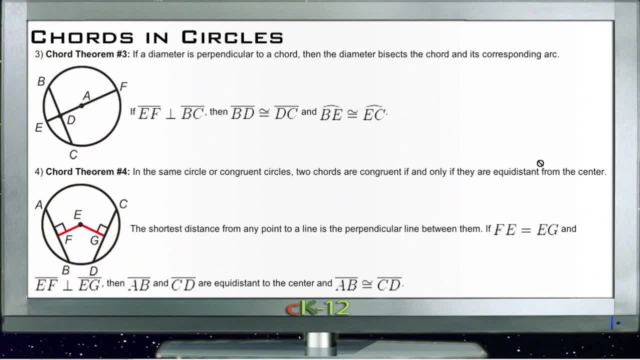 the circle. So Theorem 3 tells us that if a diameter is perpendicular to a chord, then the diameter bisects the chord and its corresponding arc. So this one is the reverse of the last one. Theorem 3 is the reverse. 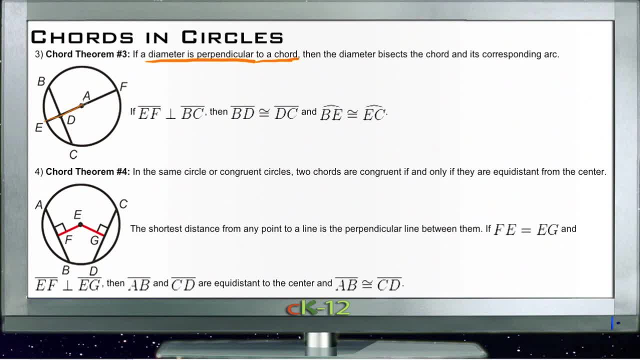 of Theorem 2. It tells us that if we have a diameter and we know that it's perpendicular to a given chord, then we also know that that diameter must have bisected that chord and of course then bisected the arc that's connected to that chord. Because the only way to get 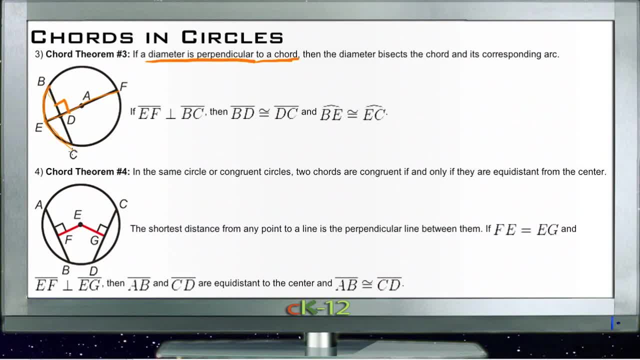 a diameter that goes through a given chord is to bisect that chord. And then, finally, Theorem 4 tells us that if we have the same circle, or two circles that are the same, two chords are congruent if they're the same distance from the center.